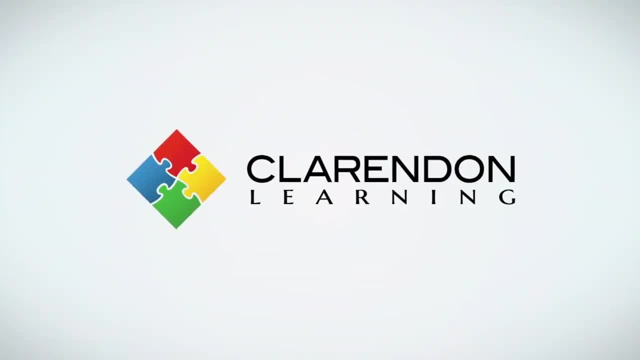 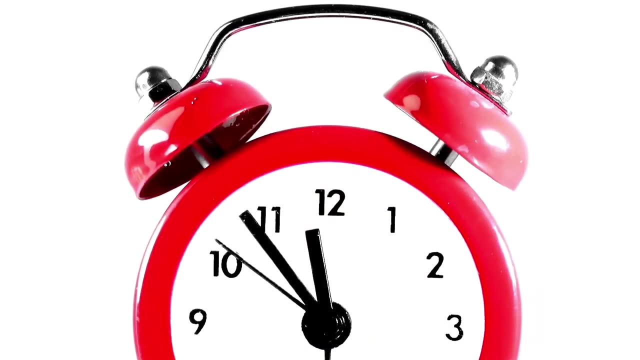 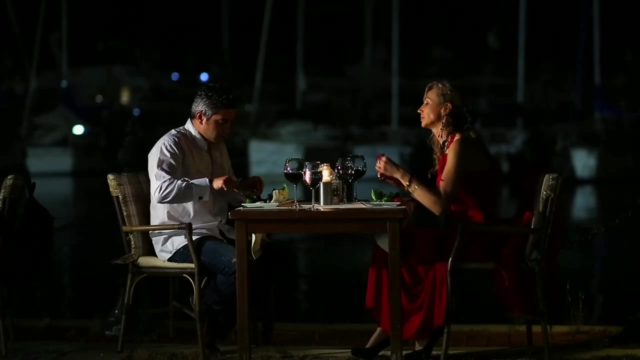 Telling Time for Kids. Every day, there are things we do at the same time. Breakfast is done in the morning, lunch is in the middle of the day and dinner is in the evening. We may get up in the morning at the same time and go to bed at the same time each night. 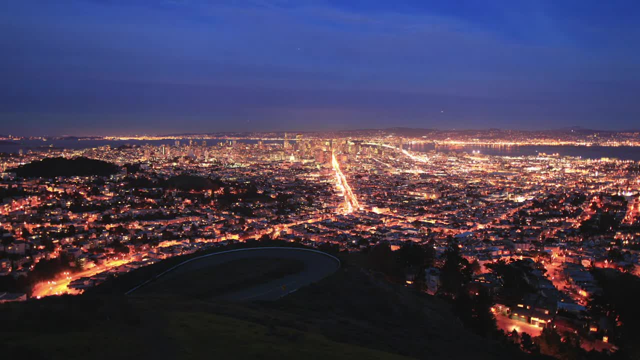 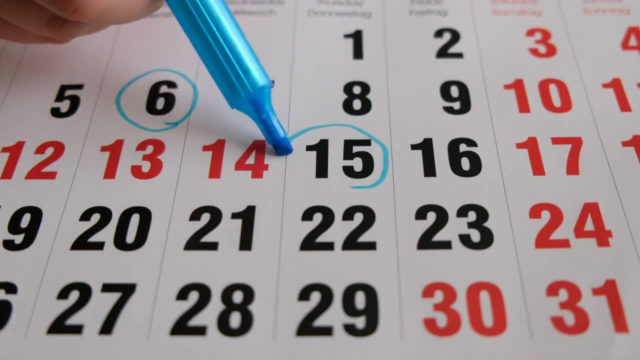 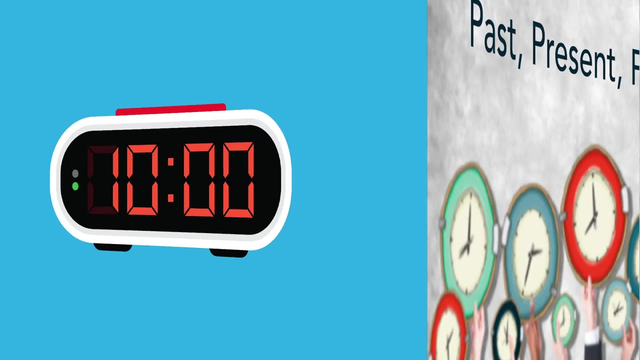 Time is an important thing. It helps us measure day and night. Time is the way we measure events that have already happened, that are happening right now or will happen. We call this the past, the present and the future. Time is measured in minutes and hours. 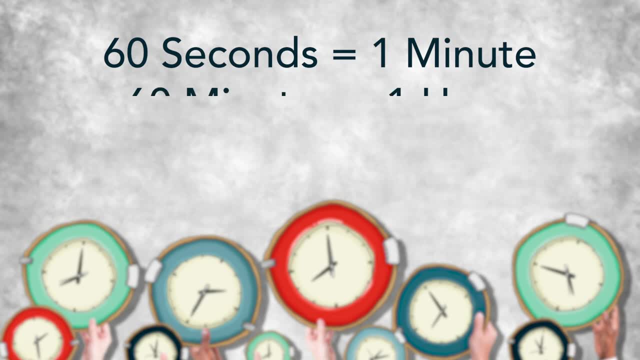 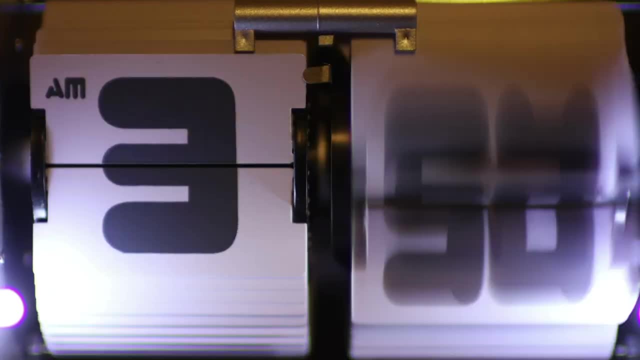 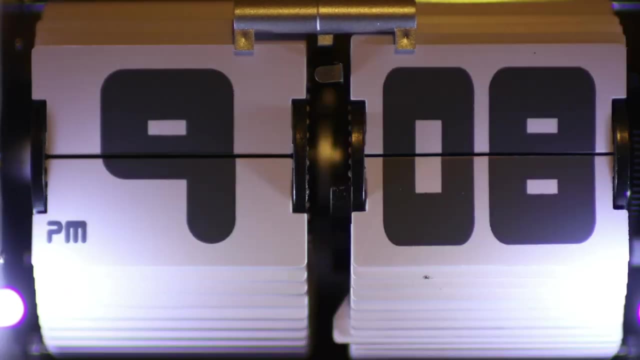 There are 60 seconds in one minute, 60 minutes make one hour And 24 hours make one day. Half or 12 of those hours make the am or morning And the other 12 hours make the afternoon and evening or pm. 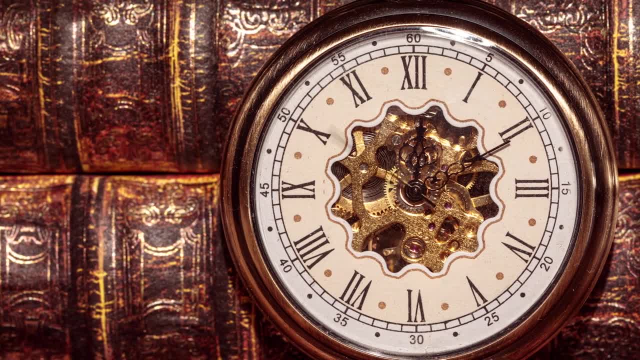 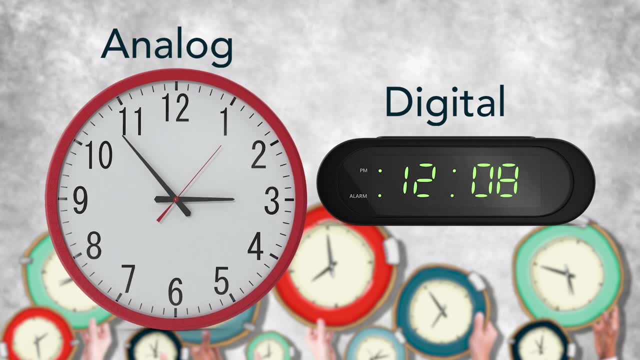 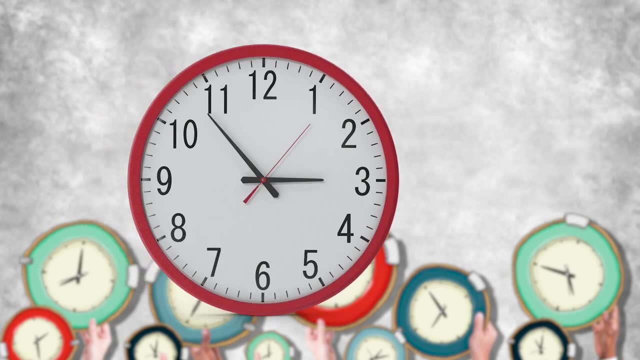 A clock is used to measure time. There are two kinds of clocks that show the time: Analog and digital. Analog clocks have moving hands- a big and a small hand- And digital clocks use numbers only. First let's talk about analog clocks. 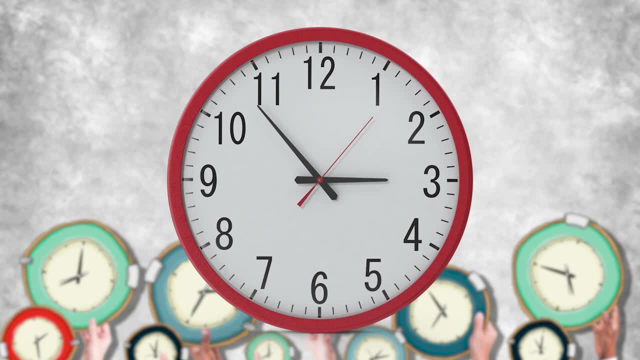 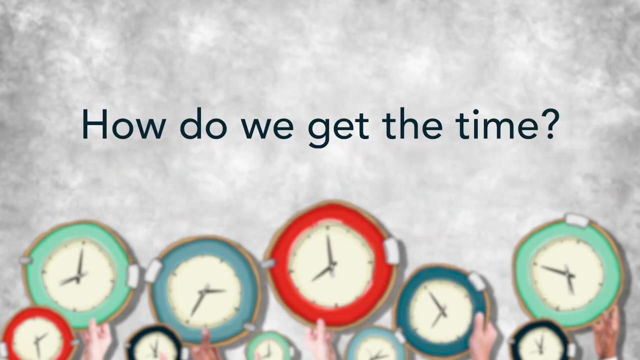 You know the ones with the hands. The numbers 1 through 12 are shown On analog clocks. The numbers represent each hour of the day. There are dashes in between each of those numbers. The dashes represent one minute each. So how do each of those dashes and numbers tell us the time? 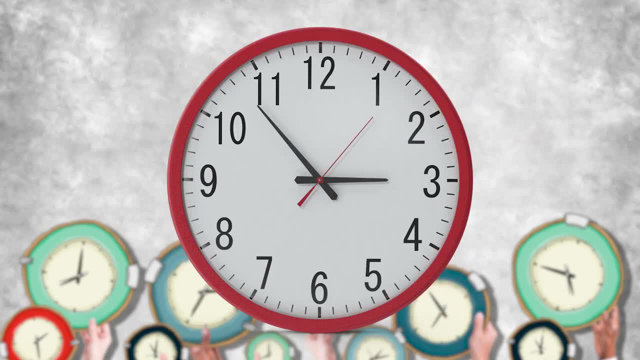 That's where the little and big hands come in. The shorter hand is called the little hand. It points to the hour. The longer hand is called the big hand. It points to the minute. Using those hands together gives us the time. 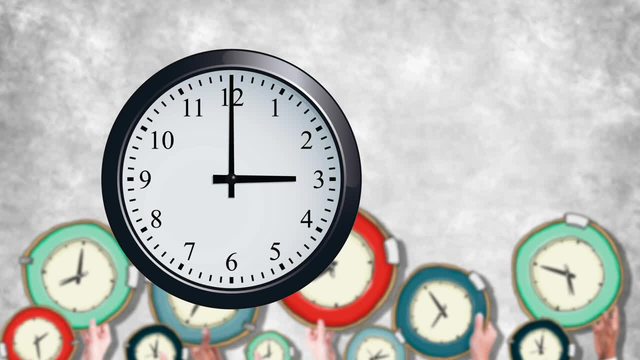 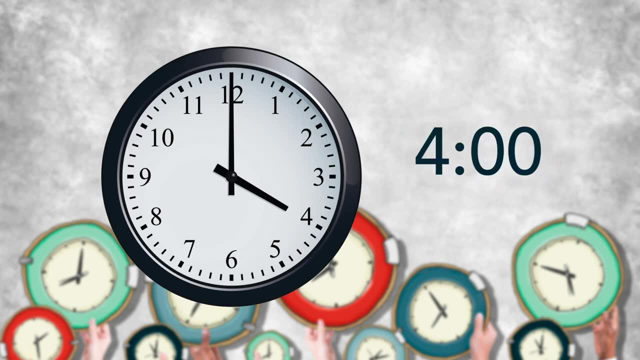 Here are some examples: If the little hand is pointing at the 3,, then we know it's 3 o'clock. If it is pointing at the 4,, then we know it's 4 o'clock. If it's pointing at 8,, 9, or 10,. 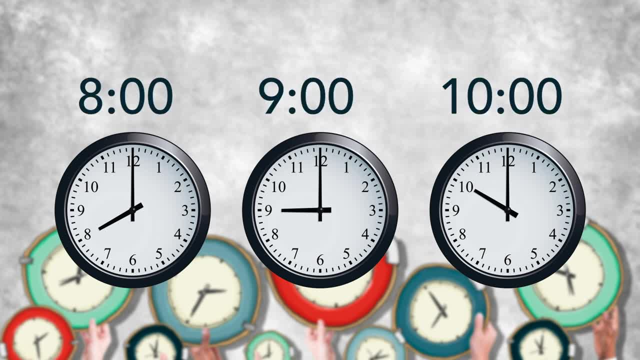 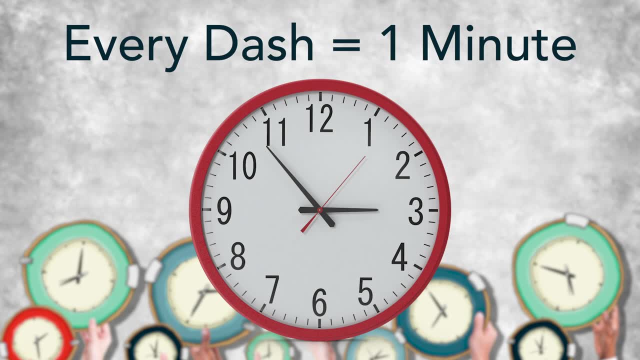 you guessed it. we know it's 8 o'clock, 9 o'clock or 10 o'clock. Can you see the dashes in between all the numbers? Each of those dashes represents one minute. From number to number, 5 minutes pass. 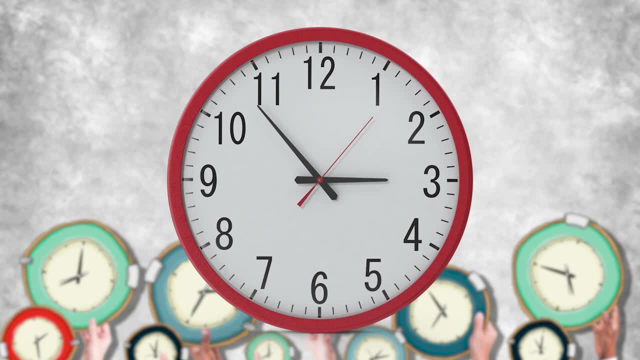 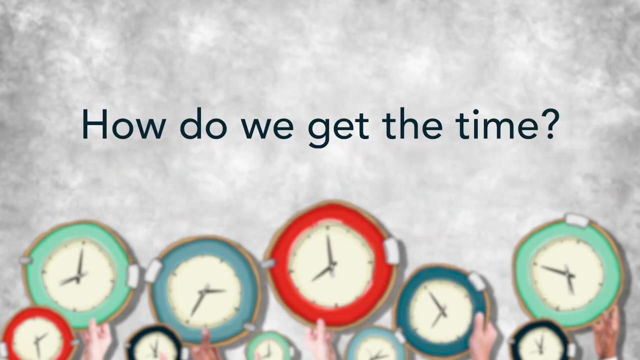 You know the ones with the hands. The numbers 1 through 12 are shown On analog clocks. The numbers represent each hour of the day. There are dashes in between each of those numbers. The dashes represent one minute each. So how do each of those dashes and numbers tell us the time? 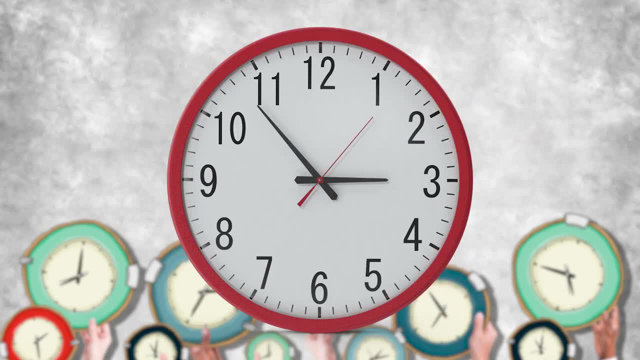 That's where the little and big hands come in. The shorter hand is called the little hand. It points to the hour. The longer hand is called the big hand. It points to the minute. Using those hands together gives us the time. 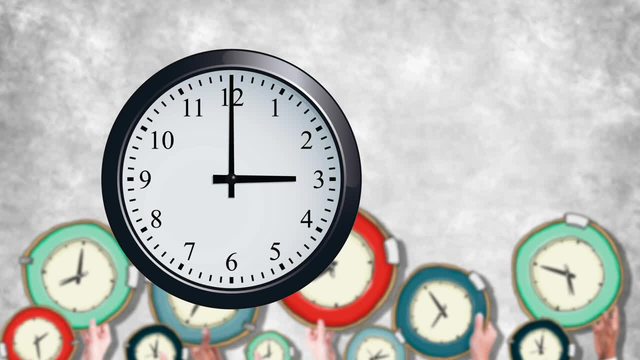 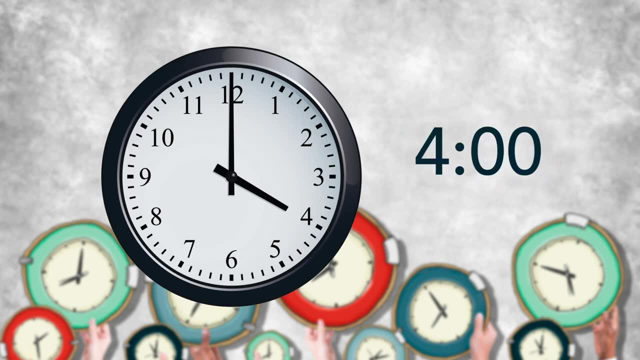 Here are some examples: If the little hand is pointing at the 3,, then we know it's 3 o'clock. If it is pointing at the 4,, then we know it's 4 o'clock. If it's pointing at 8,, 9, or 10,. 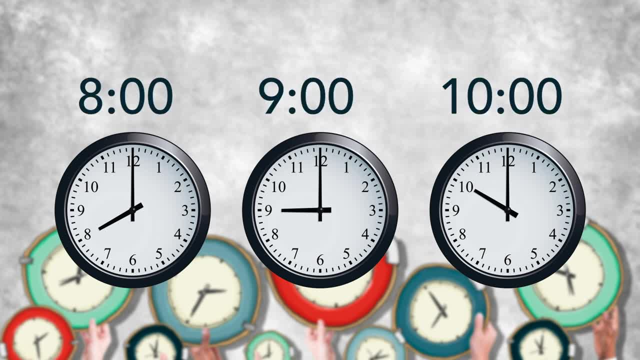 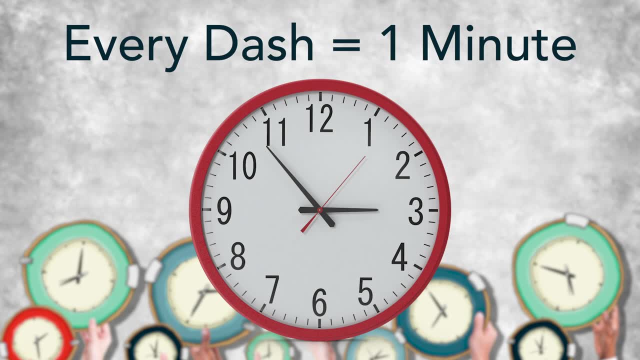 you guessed it. we know it's 8 o'clock, 9 o'clock or 10 o'clock. Can you see the dashes in between all the numbers? Each of those dashes represents one minute. From number to number, 5 minutes pass. 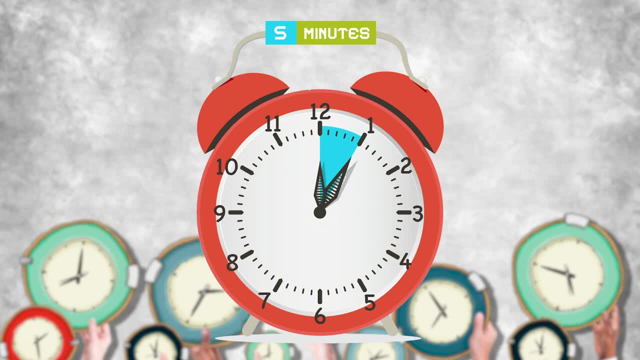 So 12 to 1 equals 5 minutes, 1 to 2 means another 5 minutes have passed, and 3 to 4 and so on. We can count each number by fives. 12 to 1 is 5.. 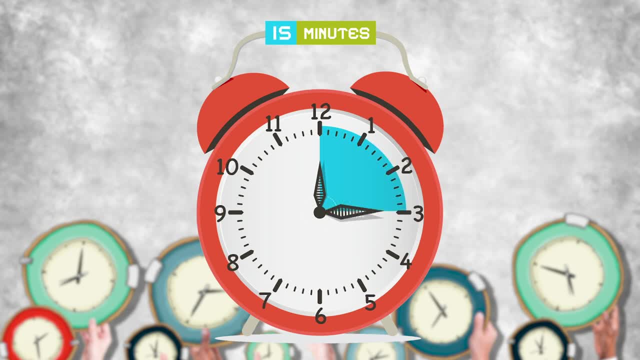 12 to 2 is 10.. 12 to 3 is 15.. Can you count the entire clock by fives? as the little hand rotates, We're going to light each number segment as you count. So here we go. 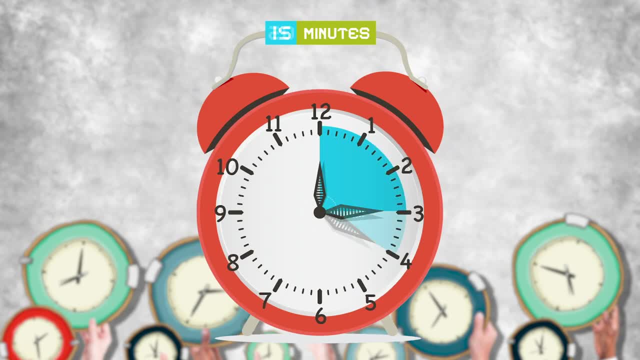 5,, 10,, 15,, 20,, 25,, 30,, 35,, 40,, 45,, 50,, 55,, 60. The last number we don't call 60. We say o'clock instead. 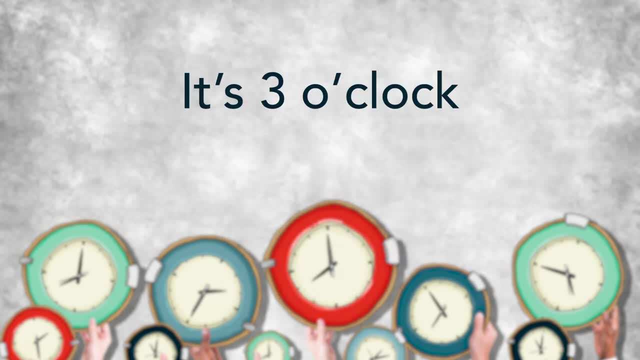 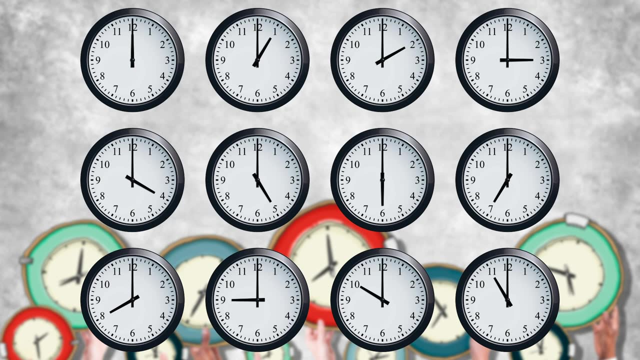 Have you ever heard someone say it's 3 o'clock or 6 o'clock? When we say o'clock, we know that the big hand is pointing at the 12. So how does the big hand help us to know what time it is? 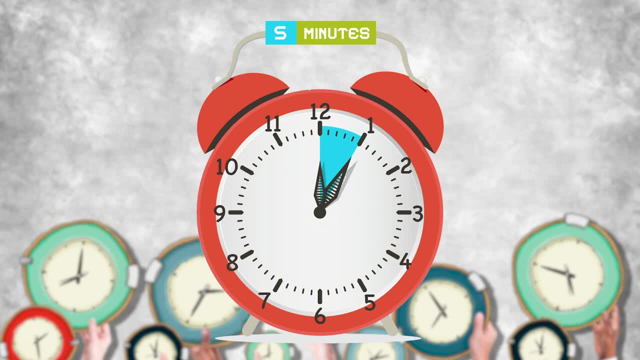 So 12 to 1 equals 5 minutes, 1 to 2 means another 5 minutes have passed, and 3 to 4 and so on. We can count each number by fives. 12 to 1 is 5.. 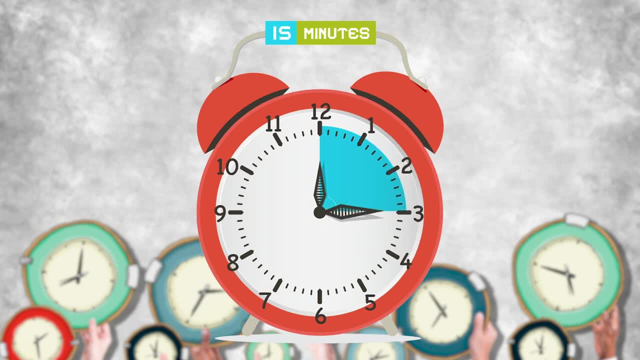 12 to 2 is 10.. 12 to 3 is 15.. Can you count the entire clock by fives? as the little hand rotates, We're going to light each number segment as you count. So here we go. 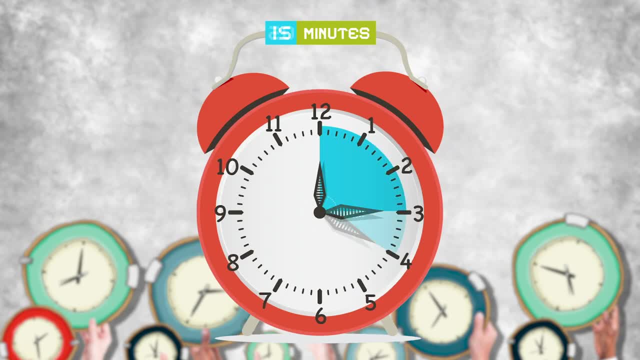 5,, 10,, 15,, 20,, 25,, 30,, 35,, 40,, 45,, 50,, 55,, 60. The last number we don't call 60. We say o'clock instead. 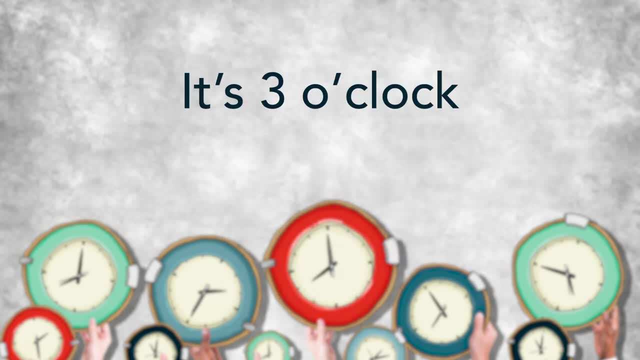 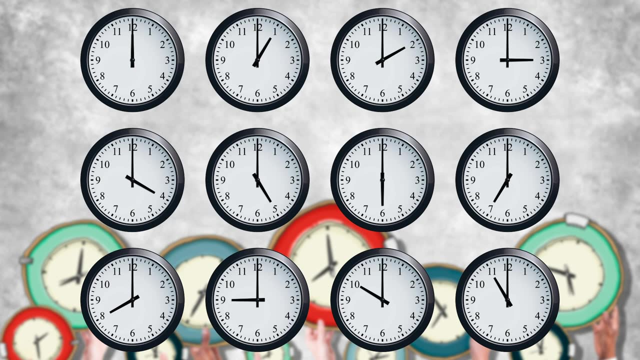 Have you ever heard someone say it's 3 o'clock or 6 o'clock? When we say o'clock, we know that the big hand is pointing at the 12. So how does the big hand help us to know what time it is? 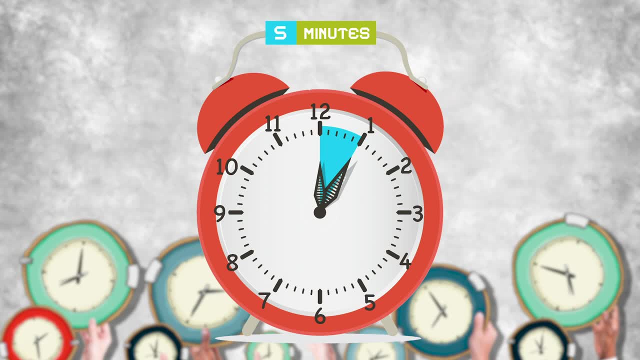 Well, when it is pointed at the 1, we know that it's 5 minutes. When it's pointed at the 2, we know it's 10 minutes. When it's pointed at the 3, it's 15 minutes. 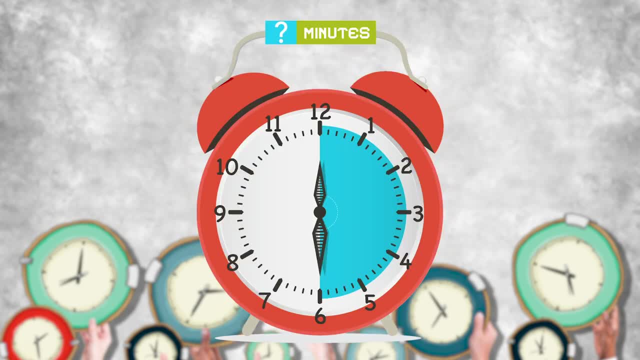 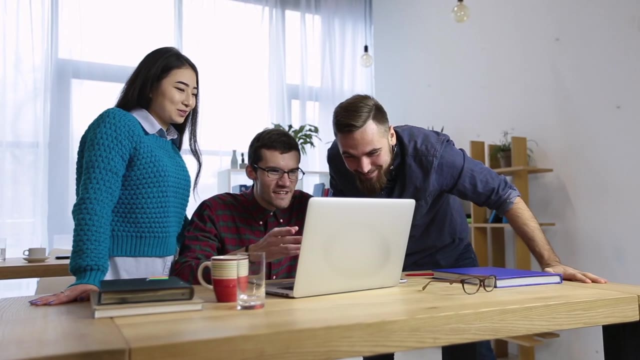 So how many minutes is it when it's pointed at the 6?? Remember, count by fives, starting at the 12.. 5, 10,, 15,, 20,, 25,, 30.. Good job, That's right. 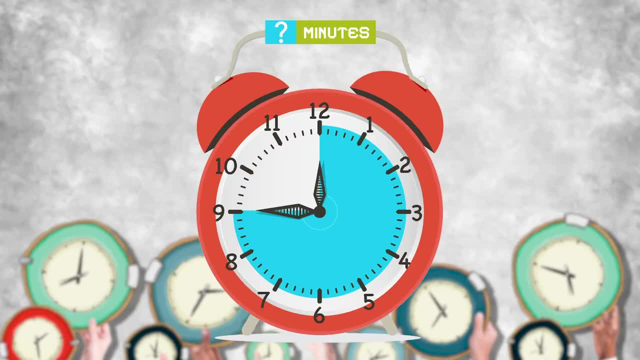 The 6 equals 30 minutes. What about the number 9 on the clock? If we know the 6 equals 30 minutes, then let's keep counting by fives from the 6. The 7 is 35 minutes and the 8 is 40 minutes. 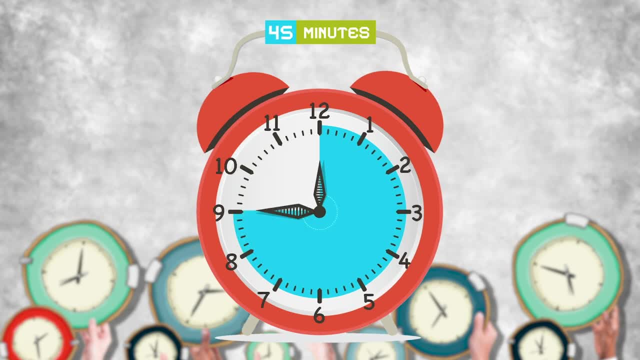 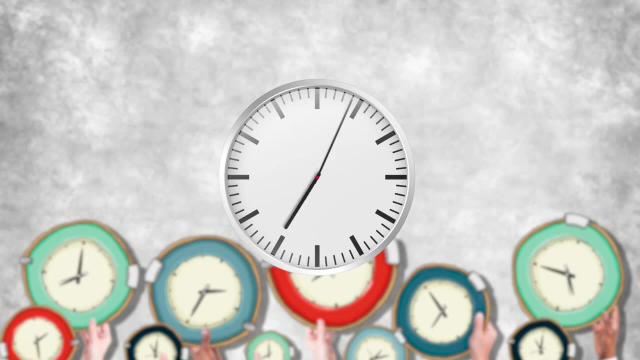 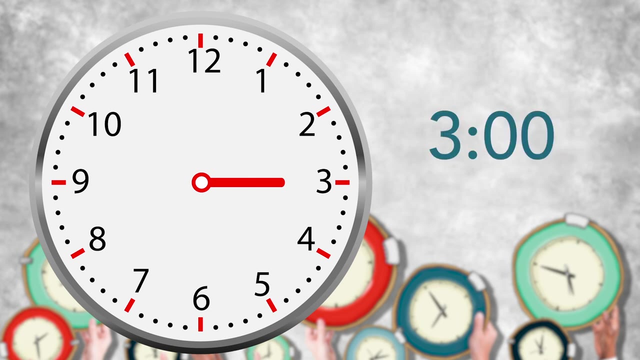 which means the 9 is 45 minutes. I think you're ready to put the two hands together and tell time. Hey, let's try it out. If the little hand is pointing to the 3,, what time is it? That's right? 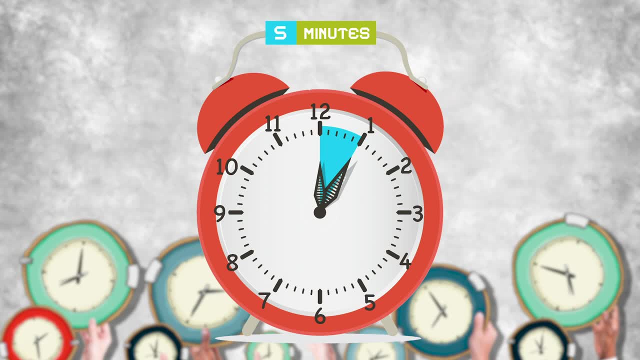 Well, when it is pointed at the 1, we know that it's 5 minutes. When it's pointed at the 2, we know it's 10 minutes. When it's pointed at the 3, it's 15 minutes. 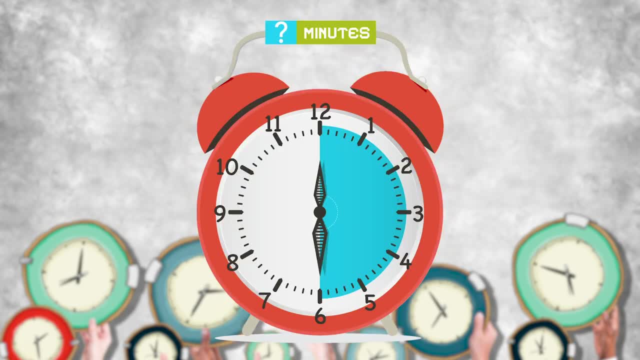 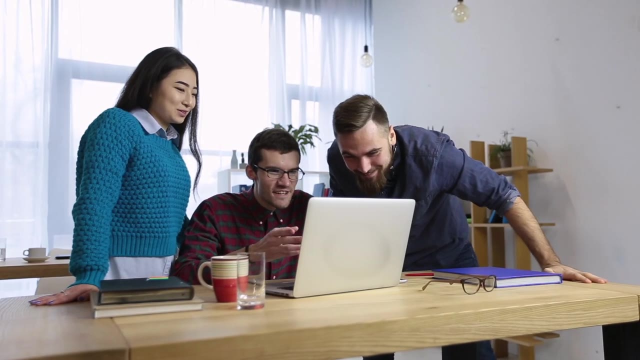 So how many minutes is it when it's pointed at the 6?? Remember, count by fives, starting at the 12.. 5, 10,, 15,, 20,, 25,, 30.. Good job, That's right. 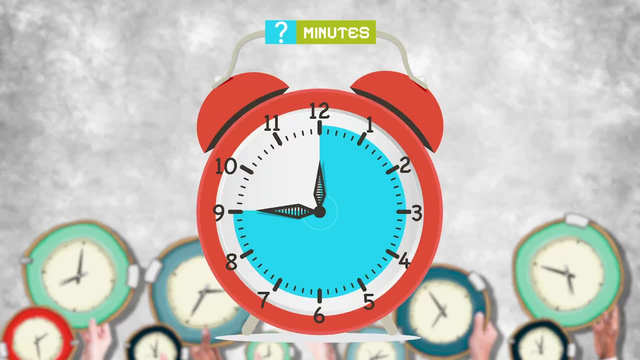 The 6 equals 30 minutes. What about the number 9 on the clock? If we know the 6 equals 30 minutes, then let's keep counting by fives from the 6. The 7 is 35 minutes and the 8 is 40 minutes. 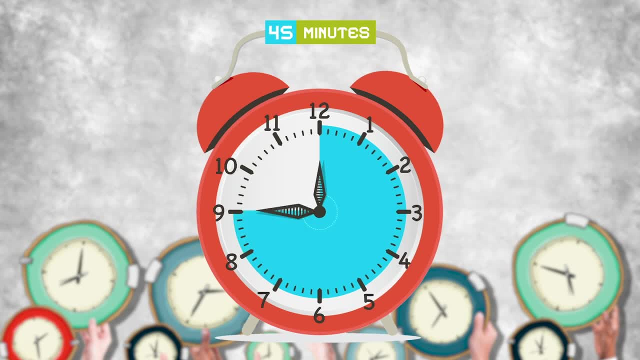 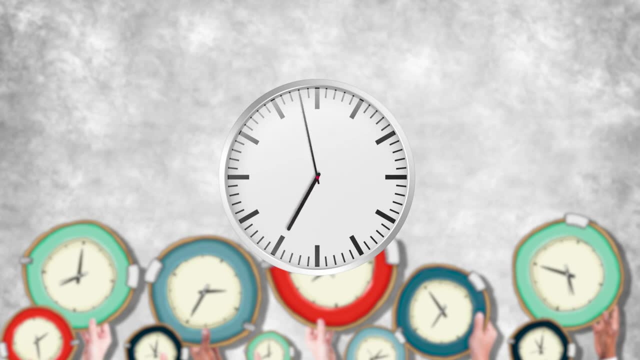 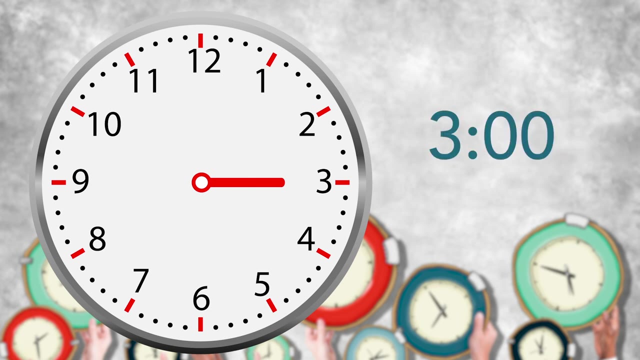 which means the 9 is 45 minutes. I think you're ready to put the two hands together and tell time. Hey, let's try it out. If the little hand is pointing to the 3,, what time is it? That's right? 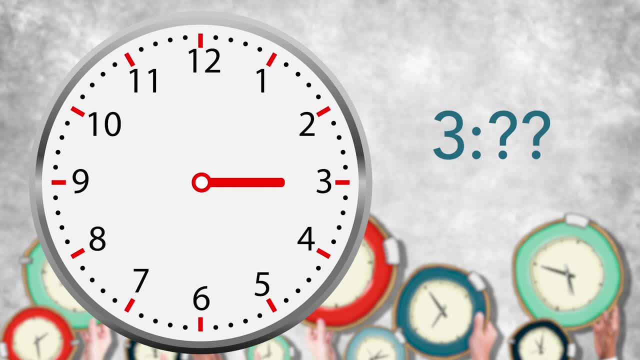 It's 3 o'clock, So now let's add the big hand. If the big hand is pointing to the 2, how many minutes is that? Hey, remember to count by fives: 5, 10.. Now all we do is put those numbers together. 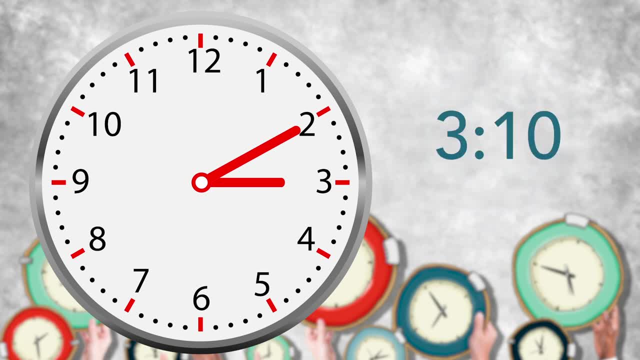 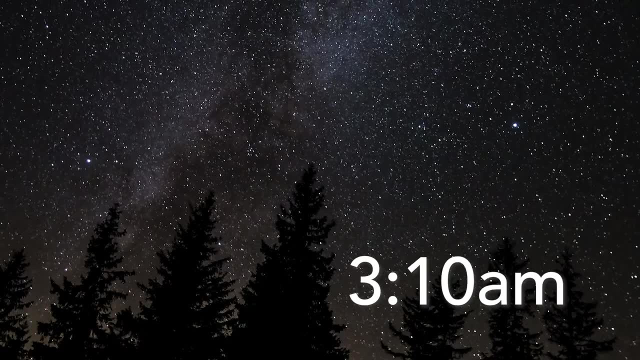 3 and 10,, or it's 310.. If it's the afternoon, then it's 310 pm. If it's very early in the morning and the sun is still not up, then it's 310 am. 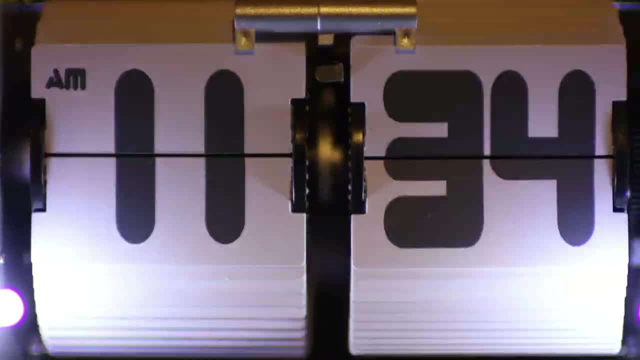 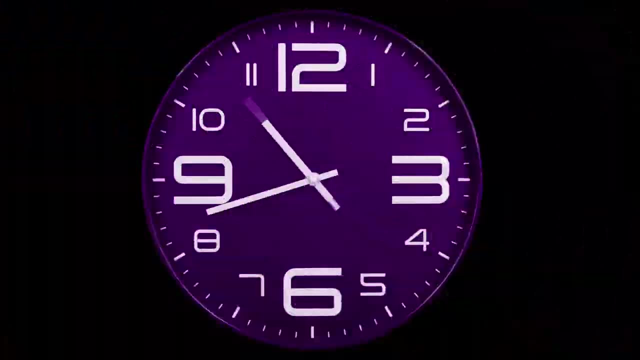 We use the same 12 numbers for am and pm. The sun helps us to know whether it's morning or evening. Let's try to see if we can figure out some more times on our clock If the little hand is pointing at the 5,. 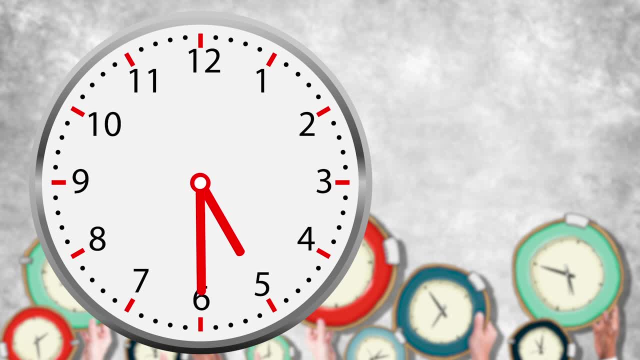 and the big hand is pointing at the 6,. what time is it? We know that the first number is 5, so now all we need to do is count by fives to find out the rest of the time: 5,, 10,, 15,, 20,, 25,, 30. 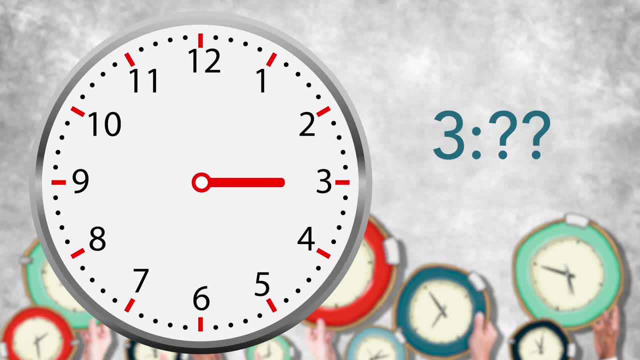 It's 3 o'clock, So now let's add the big hand. If the big hand is pointing to the 2, how many minutes is that? Hey, remember to count by fives: 5, 10.. Now all we do is put those numbers together. 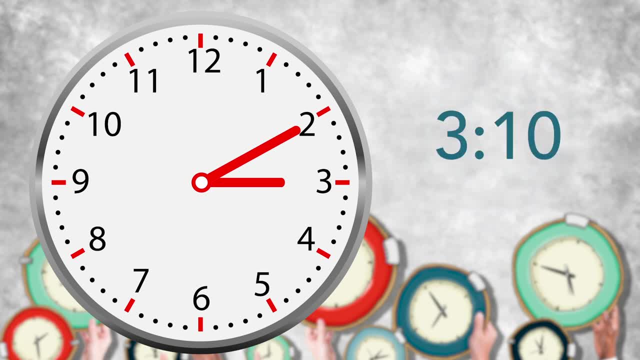 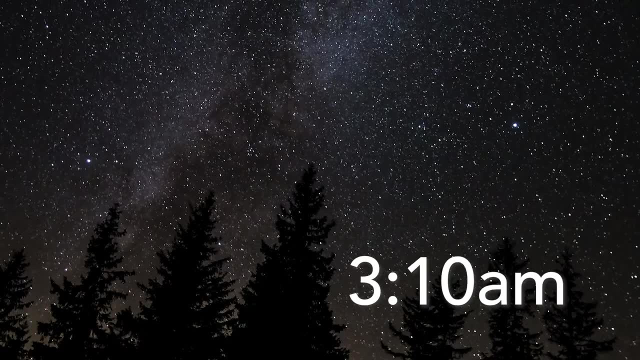 3 and 10,, or it's 310.. If it's the afternoon, then it's 310 pm. If it's very early in the morning and the sun is still not up, then it's 310 am. 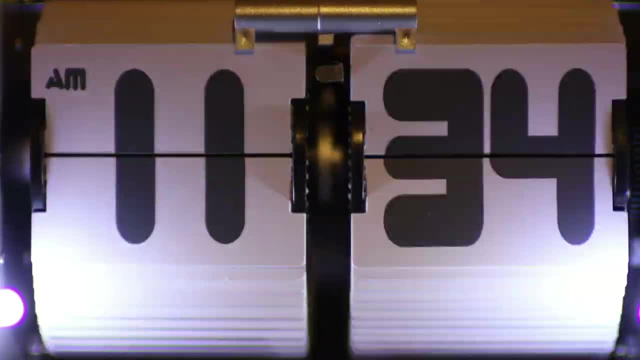 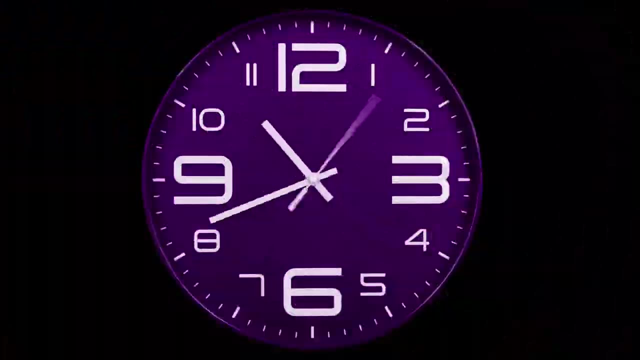 We use the same 12 numbers for am and pm. The sun helps us to know whether it's morning or night. Let's try to see if we can figure out some more times on our clock If the little hand is pointing at the 5. 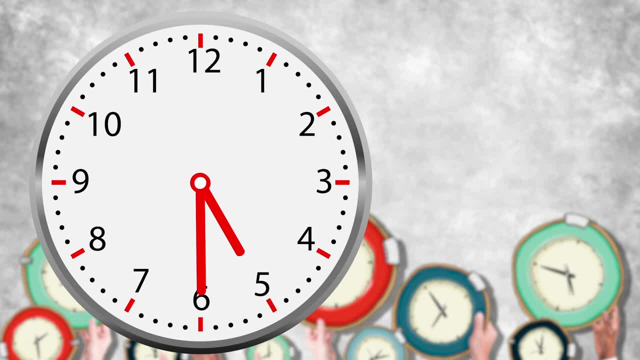 and the big hand is pointing at the 6,. what time is it? We know that the first number is 5, so now all we need to do is count by fives to find out the rest of the time: 5,, 10,, 15,, 20,, 25,, 30. 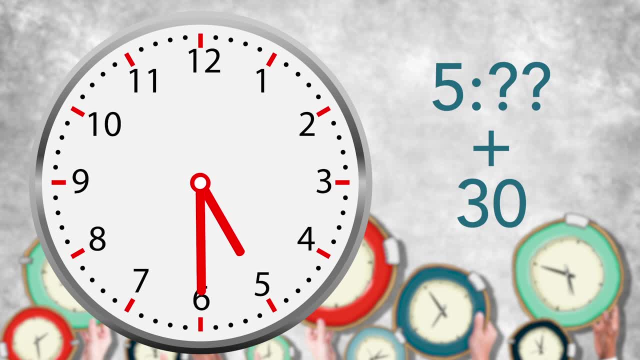 When we put the 5 and the 30 together, what time does that become? Did you say 5.30?? If you did, you're right. Well done. At 5.30 pm you might be eating dinner. 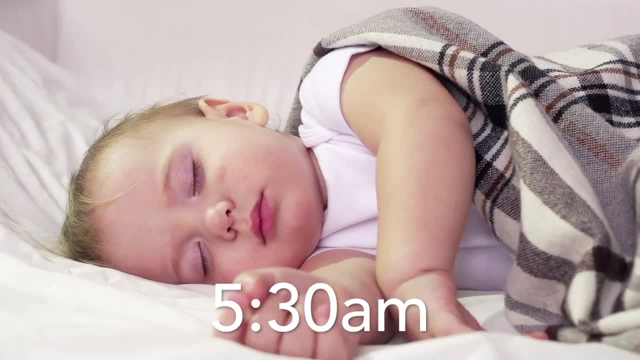 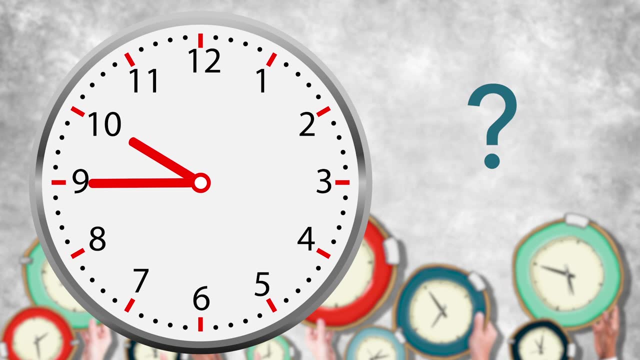 At 5.30 am, you might be asleep. How about if the little hand is pointing at the 10 and the big hand is pointing at the 9?? Can you figure that out? Did you get 10.45?? If you did, you know how to tell time? 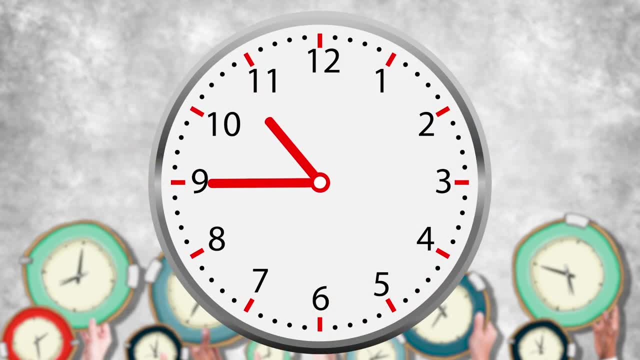 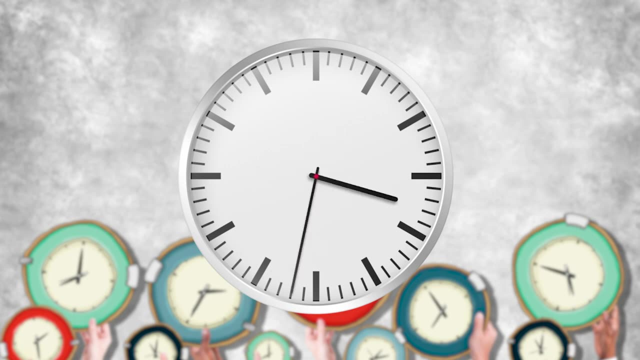 Let's look closely at this time on the clock. Do you notice that when the time on the analog clock shows 10.45, that the little hand is closer to the 11 than the 10?? That's because the little hand moves just like the big hand does. 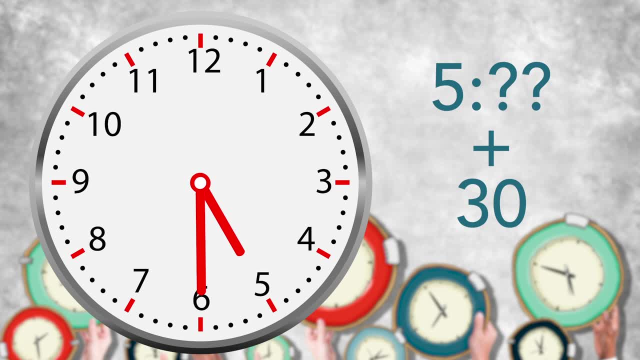 When we put the 5 and the 30 together, what time does that become? Did you say 5.30?? If you did, you're right. Well done. At 5.30 pm you might be eating dinner. 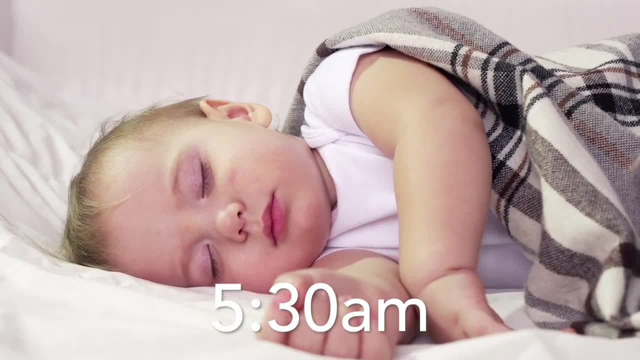 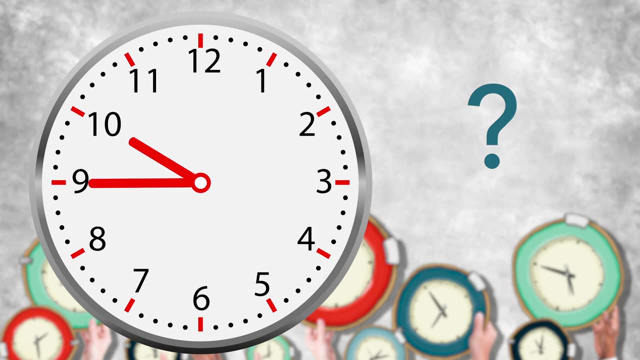 At 5.30 am you might be asleep. How about if the little hand is pointing at the 10, and the big hand is pointing at the 9?? Can you figure that out? Did you get 10.45?? 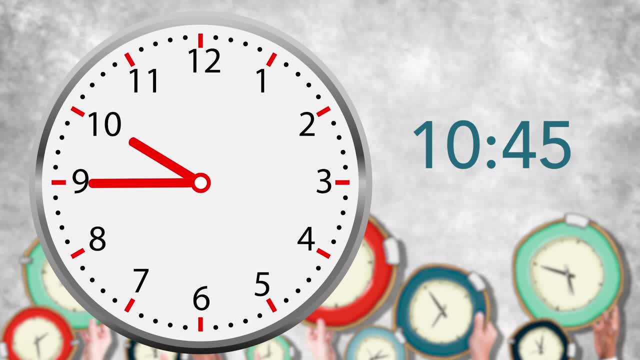 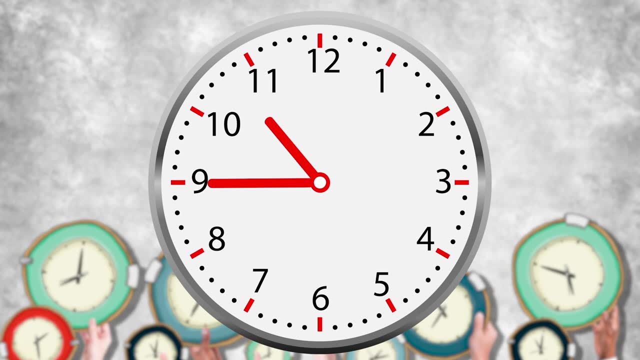 If you did, you know how to tell time. Let's look closely at this time on the clock. Do you notice that when the time on the analog clock shows 10.45, that the little hand is closer to the 11 than the 10?? 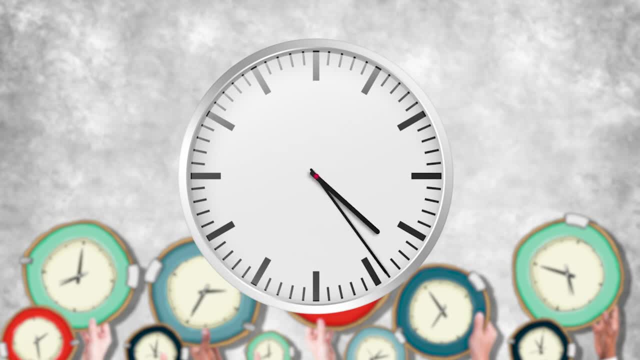 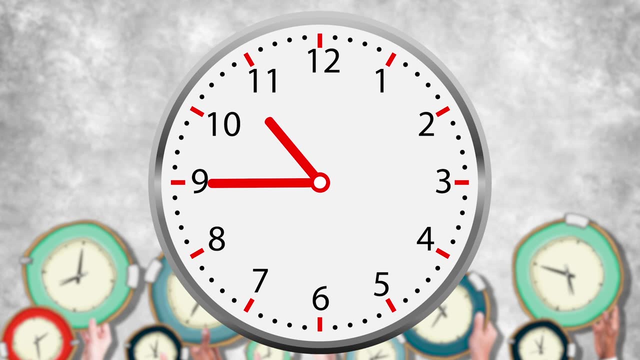 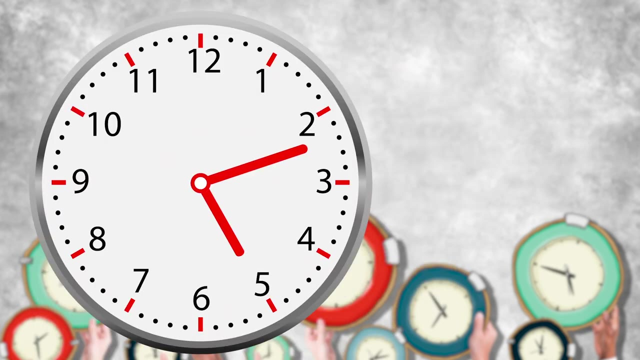 That's because the little hand moves just like the big hand does, It just moves slower. It's closer to the 11, at 10.45, because it's almost 11 o'clock. The same thing happens with the numbers When the little hand is in between numbers. 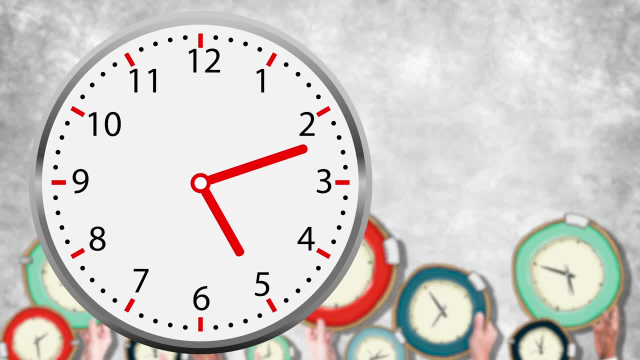 and pointing to a dash. we will need to count the dashes after a number to know exactly what time it is. If the little hand is pointing at the 5, and the big hand is pointing at two dashes past the 2,, then we would count by 5,. 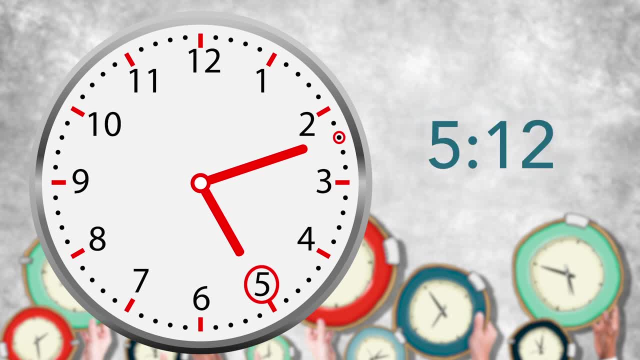 and then add 2 to find out that it's 5.12.. How about if the little hand is pointing at the 4, and the big hand is pointing at three dashes past the 6? That would mean it would be 4.30 plus 3,. 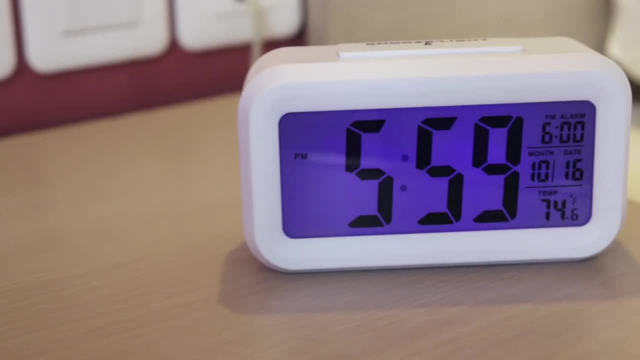 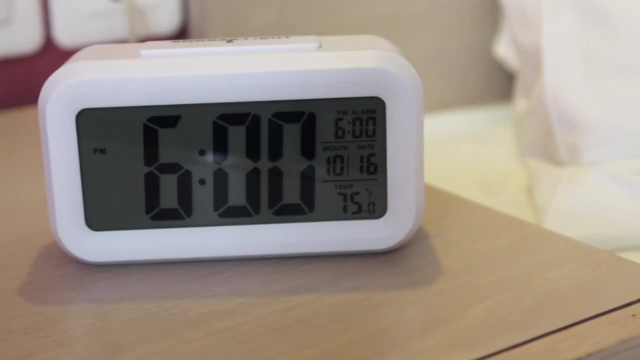 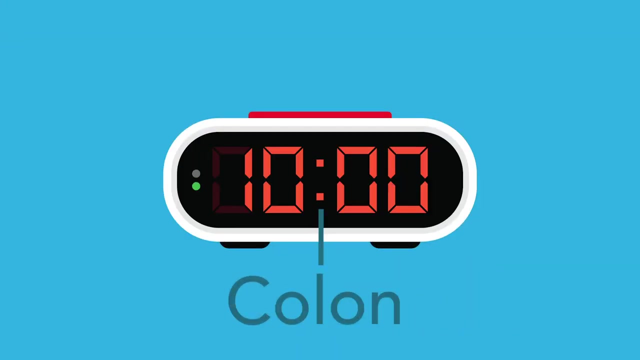 or 4.33.. Now that you know how to tell time on an analog clock, let's look at a digital clock. These clocks do not have hands. They show the time with the numbers separated by a colon. See this: This here is a colon. 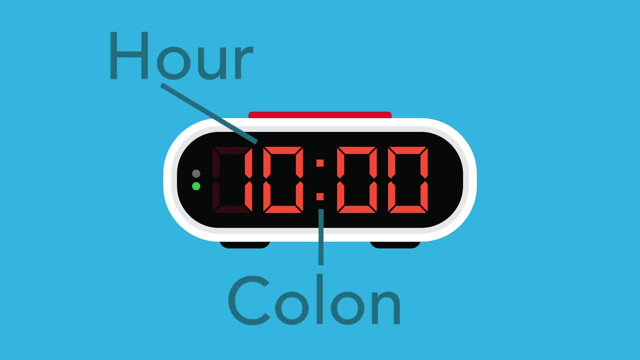 The number on the left side of the colon is the hour. The number on the right side of the colon shows the minutes. On this clock. the number 3 is shown on the left, then the colon and now the number 40.. 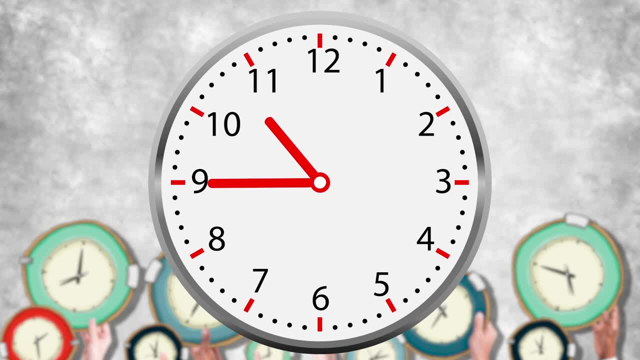 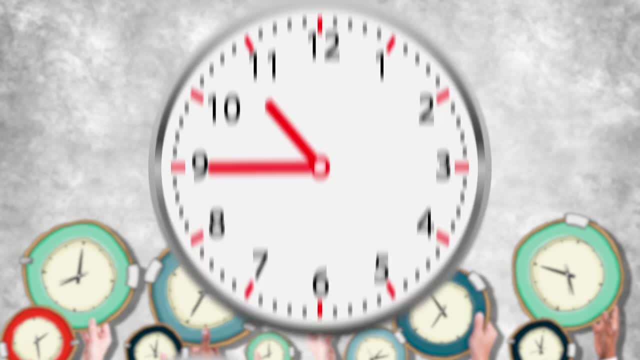 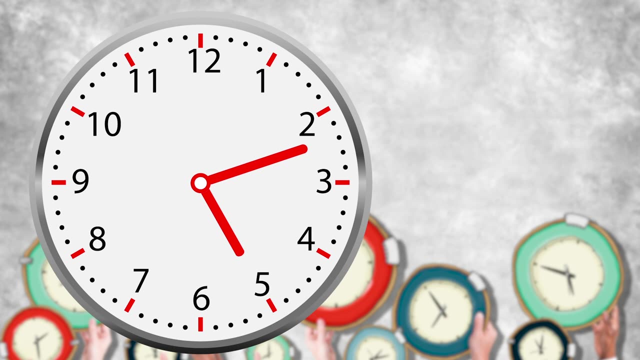 It just moves slower. It's closer to the 11 at 10.45 because it's almost 11 o'clock. The same thing happens with the numbers. When the little hand is in between numbers and pointing to a dash, we will need to count the dashes after a number. 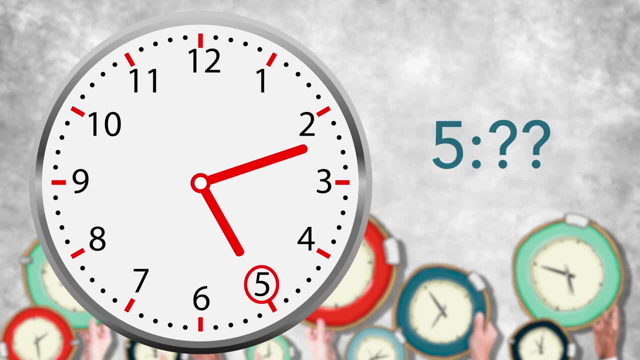 to know exactly what time it is. If the little hand is pointing at the 5 and the big hand is pointing at two dashes past the 2, then we would count by 5 and then add 2 to find out that it's 5.12.. 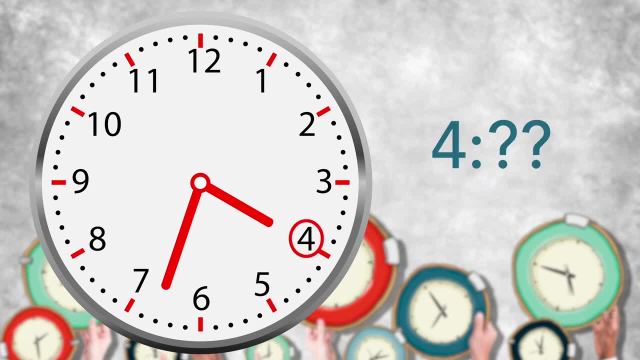 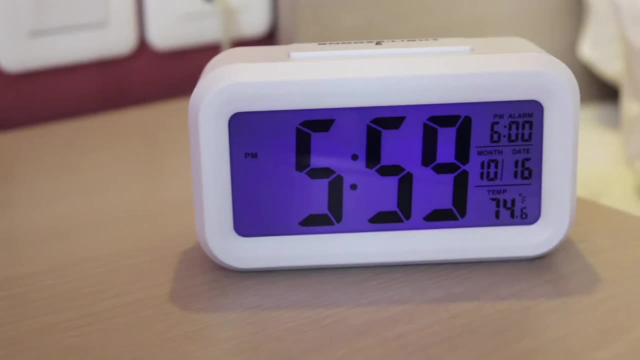 How about if the little hand is pointing at the 4 and the big hand is pointing at three dashes past the 6?? That would mean it would be 4.30 plus 3 or 4.33.. Now that you know how to tell time on an analog clock. 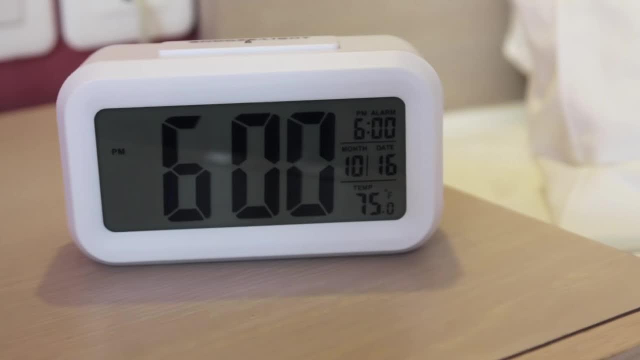 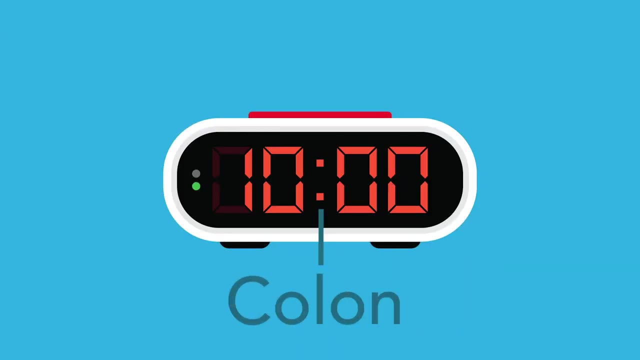 let's look at a digital clock. These clocks do not have hands. They show the time, with the numbers separated by a colon. See this: This here is a colon. The number on the left side of the colon is the hour. The number on the right side of the colon shows the minutes. 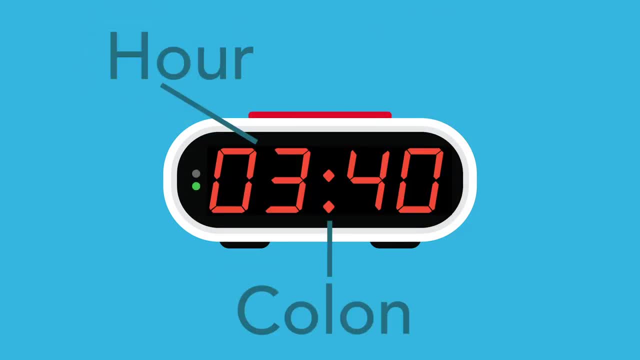 On this clock, the number 3 is shown on the left, then the colon and now the number 40. That means it's 3.40.. Let's look at another clock. This clock shows the number 7, followed by the colon. 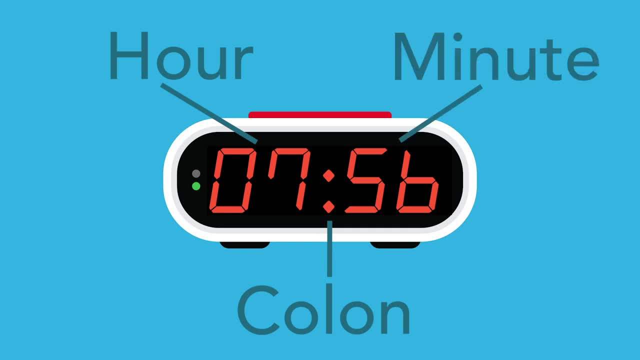 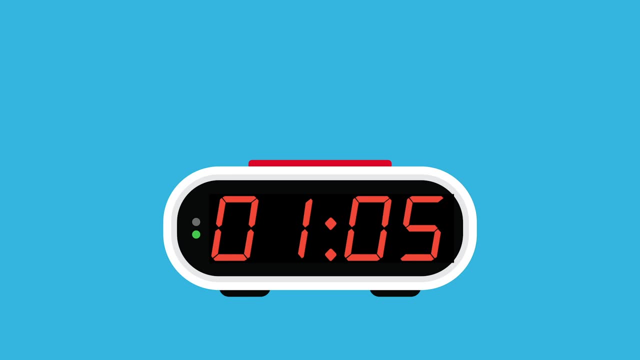 then the number 56.. That means it's 7.50.. That means it's 7.56.. How about this clock? On this clock, the time would be 1.05.. When there is a zero after the colon and before the next number. 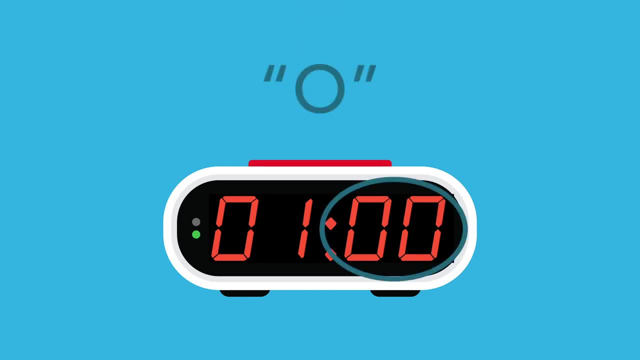 we say O instead of zero. Remember, when there are two zeros after the first number, we say O'clock, But if there is a number after the zero, then we say O and then the number or 1.05.. If the clock reads 1,. 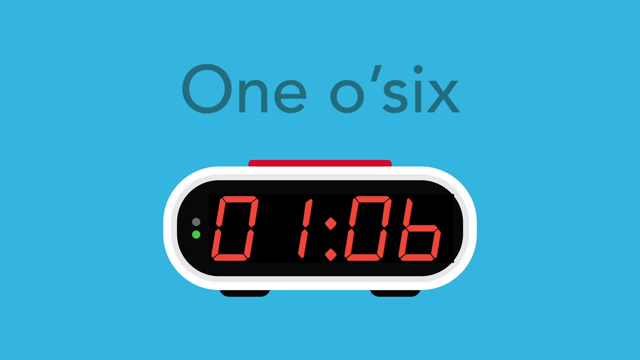 and then a zero and a 6,, then we would say 106, then 107,, then 108, and 109, until it gets to the number 10.. Now let's put the analog and digital clocks side by side. 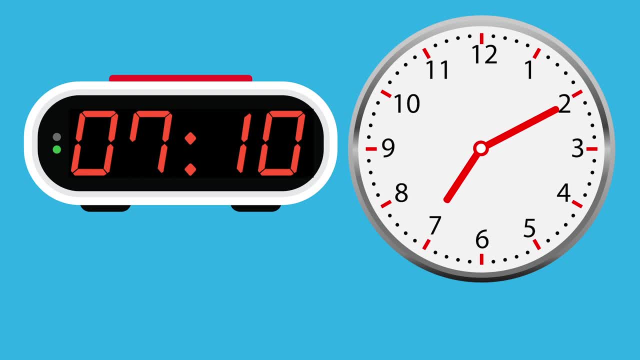 and let's see if you can tell what time it is. If you said 7.10,, then you're right. Hey, how about this one? Did you say 11.10?? Did you say 11.10?? Wow? 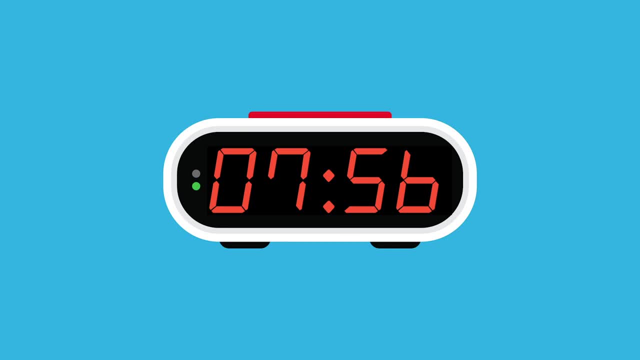 That means it's 3.40.. Let's look at another clock. This clock shows the number 7, followed by the colon, then the number 56. That means it's 7.50.. That means it's 7.56.. 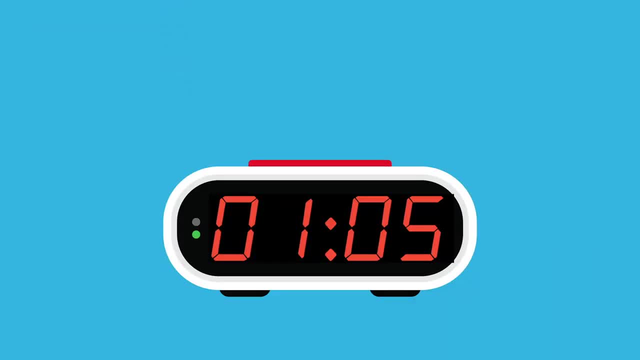 How about this clock? On this clock, the time would be 1.05.. When there is a zero after the colon and before the next number, we say O instead of zero. Remember when there are two zeros after the first number. 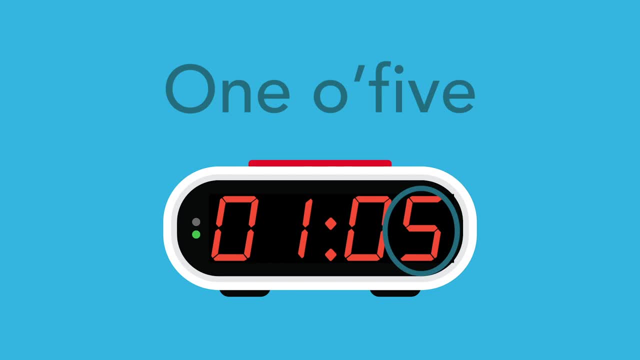 we say O'clock, But if there is a number after the zero, then we say O and then the number or 1.05.. If the clock reads 1,, then we say 0.5.. If the clock reads 1,, then we say 0.5.. 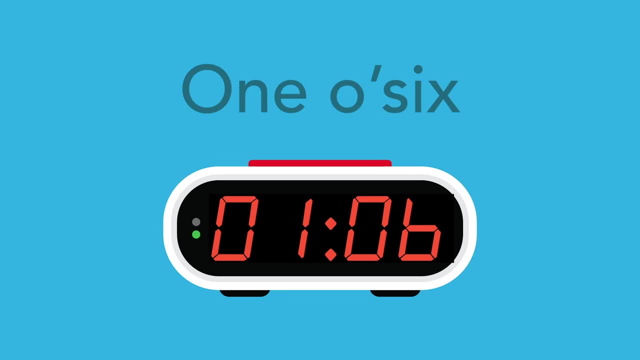 If the clock reads 1, and then a zero and a 6,, then we would say 1.06,, then 1.07,, then 1.08, and 1.09, until it gets to the number 10.. 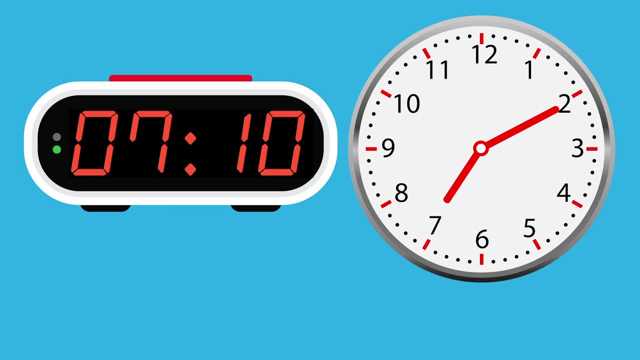 Now let's put the analog and digital clocks side by side and let's see if you can tell what time it is. If you said 7.10,, then you're right. Hey, how about this one? Did you say 11.10?? 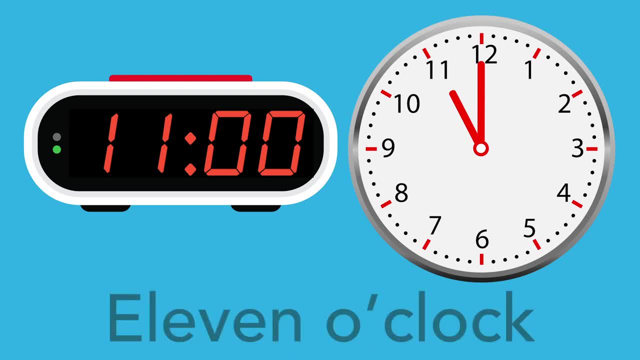 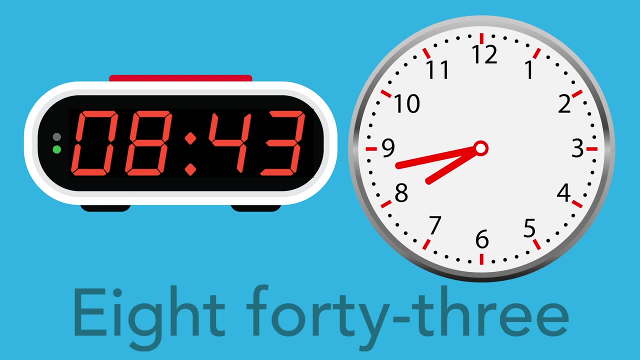 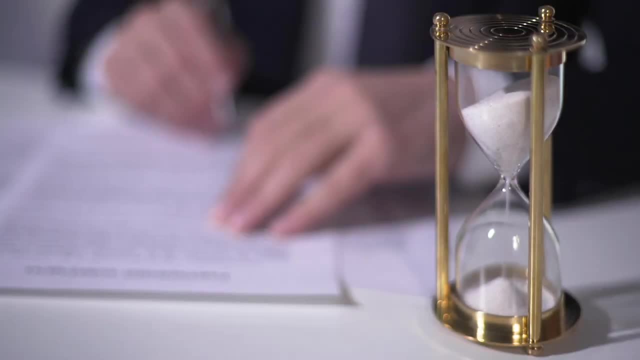 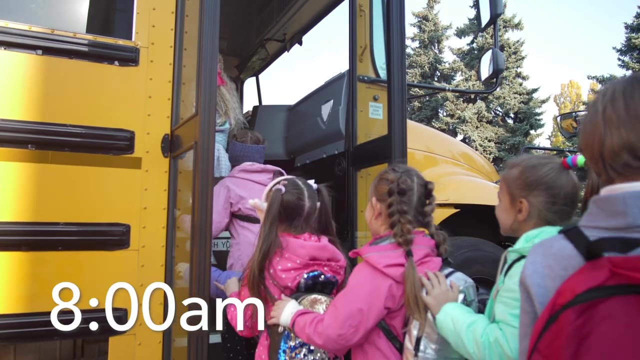 You just learned how to tell time. Learning how to tell time is a good thing because we use time to measure all sorts of things. At 8 am you may get up in the morning to go to school. At 8 pm you may be getting ready for bed. 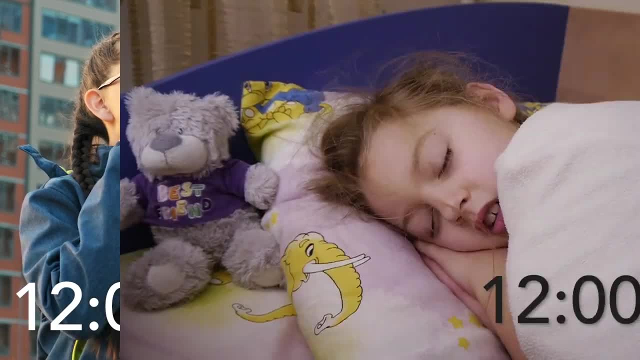 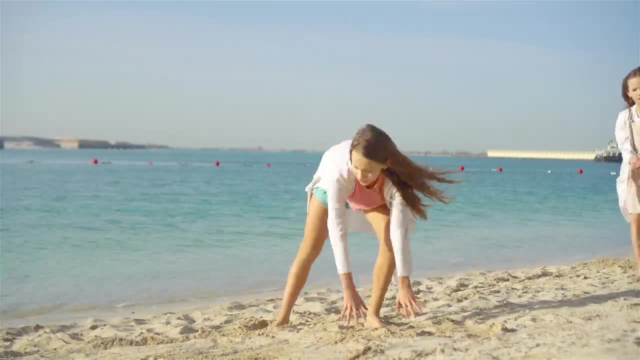 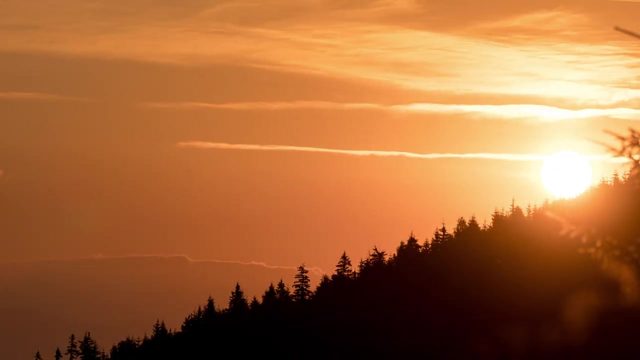 12 pm might be your lunch time, while 12 am you're probably fast asleep. Time seems to go quickly when we are doing something we enjoy, and slow down when we're doing something we might not like. No matter what you're doing, time keeps moving and never stops. 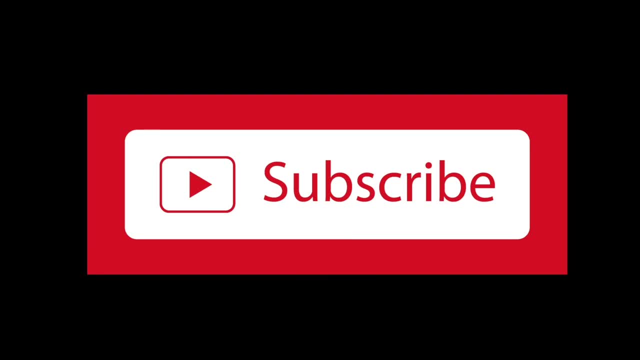 Thanks for following Clarendon Learning. Be sure to subscribe For more fun videos. visit ClarendonLearningcom. Thanks for following Clarendon Learning. Be sure to subscribe For more fun videos. visit ClarendonLearningcom For more free resources. check us out at ClarendonLearningorg.